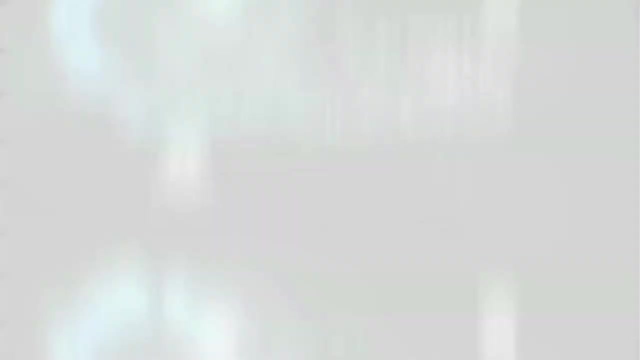 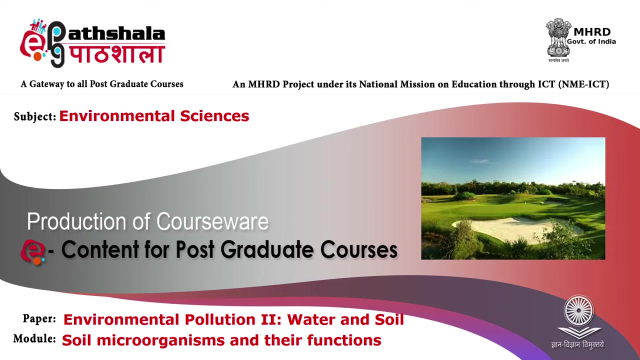 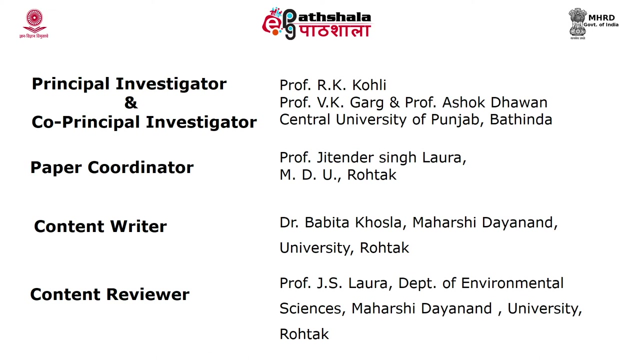 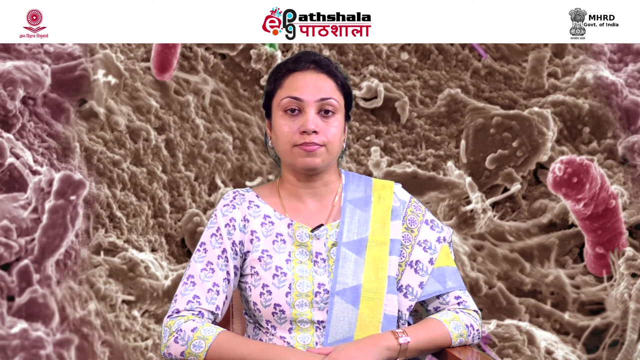 Hello students, welcome to EPG Partshala. Today we will discuss the module Soil: Microorganisms and their functions. Microorganisms, they are small, microscopic organisms which are present all around us: in water, in air and in soil. Soil is the most favorable medium for the microorganism. 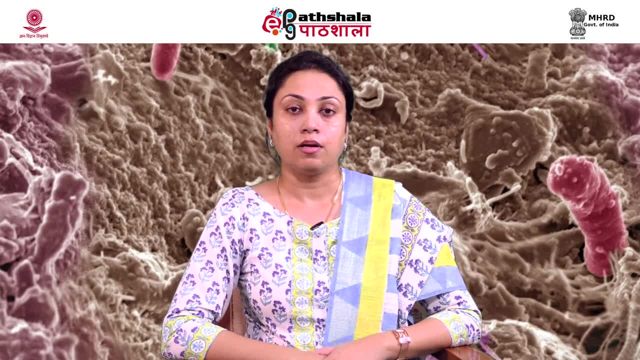 as it is rich in the organic matter. The vast variety of the microorganisms present in the soil include bacteria, fungi, viruses, protozoa and actinomycetes In the soil. these microorganisms, they play a very diverse role. They are acting as the decomposers in the soil for the sustainability. of the soil ecosystem. They are degrading, or we can say decomposing, the living or the dead organic matter which is present in the soil and make it available to the plant In the soil. they are also acting as nitrogen fixers, because they are fixing the atmospheric nitrogen into ammonia. 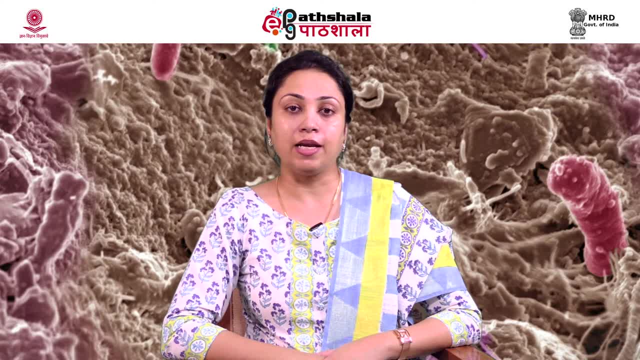 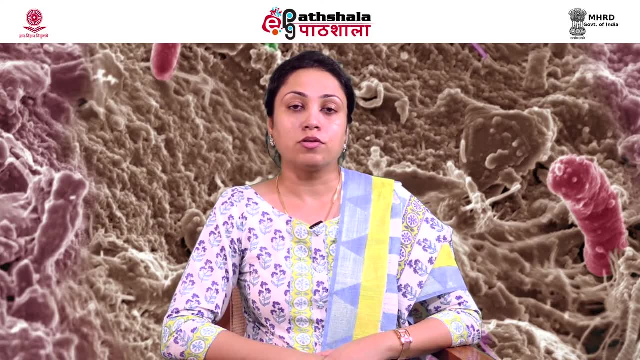 nitrites and nitrates, and these forms are readily available to the plant. These bacteria in the soil also act as the phosphorus solubilizers and they are solubilizing the complex form of the phosphates with the calcium, aluminium and iron into the available form which can be readily utilized. 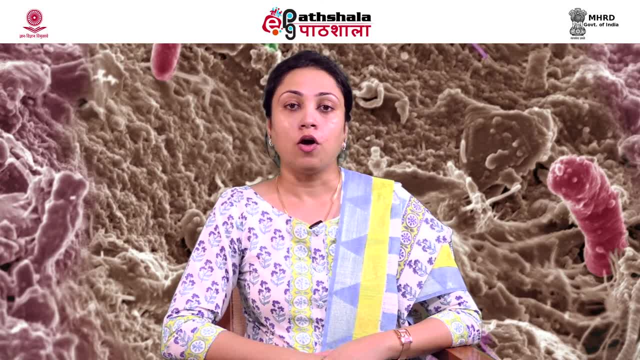 Because of the activity of the bacteria as a nitrogen fixer and as phosphorus solubilizer, they are also commercialized as biofertilizers. These bacteria not only acting as the biofertilizers, they are also producing certain phytohormones, as well as certain other molecules which will 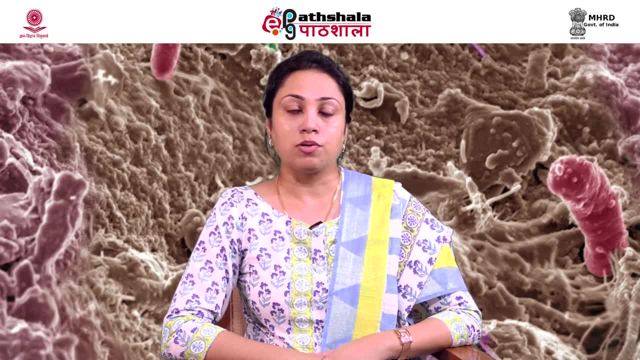 regulate the growth of the plants. That's why they are also having the plant growth promoting role present in the rhizosphere area of the plant. in addition to this, the bacteria, they are also acting as the disease suppressors and this activity of the bacteria is commercialized as. 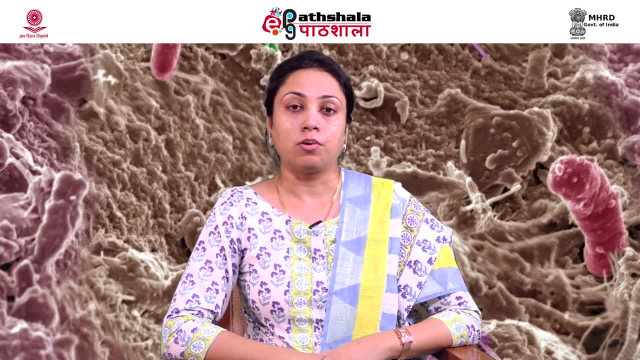 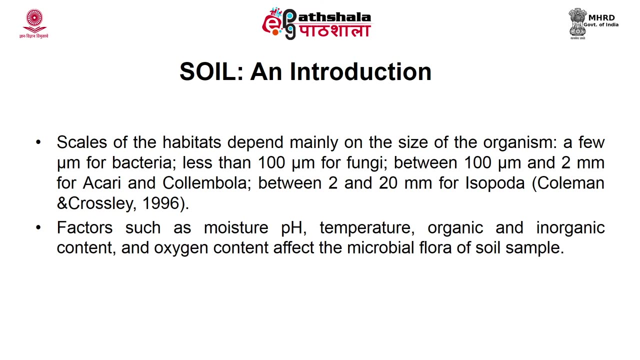 their potential in biocontrol agents. so in this module today, we will discuss the various kinds of bacteria which are present in the soil and their role in maintaining the soil ecosystem. soil is the natural and dynamic medium for the growth of land plants, and it is an important factor which influences the productivity of our planet's ecosystem. 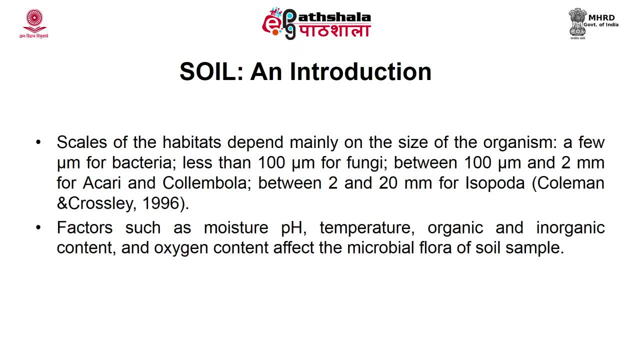 a mass of mineral particles alone do not constitute soil but it contains also air water dead organic matter and various types of living organisms the formation of a soil is influenced by the kind of organisms present in the soil的自然 而地球運用者 将lies烜 pulp � habitual soil- Information Warming substances of all organic matter, riposte, Fibrds. 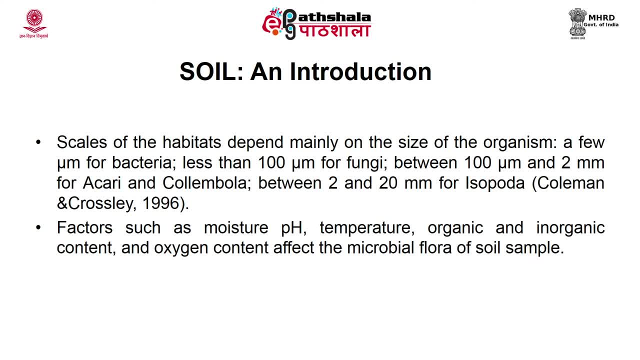 pertama但是 Elsa, which is the most信心伀生物 which is known from the nature, both in terms of 在 issula and plus in terms of tons and��。 in the soil, the climate, topography and the parent material of that area, as well as the time period. 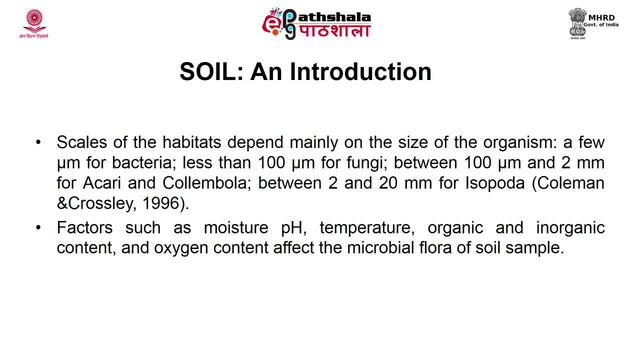 true. soils are influenced, modified and supplemented by living organisms and soil contain different type of microorganisms, including bacteria, actinomycetes, fungi, algae and viruses, the plants and animals. they aid in the development of the soil through the addition of organic matter microorganisms, mainly fungi and bacteria. they decompose this organic matter into semi-soluble. 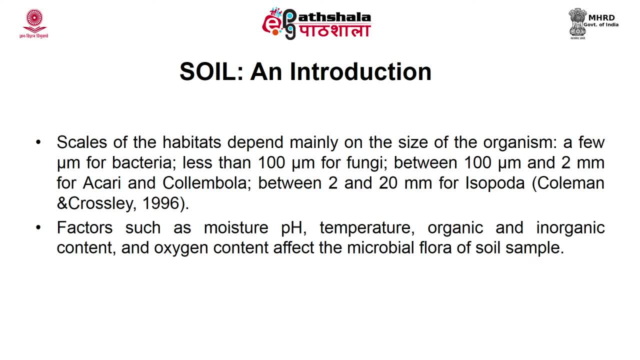 chemical substance which is known as humus, larger soil microorganisms like earthworms, beetles and termites. they also vertically distribute this humus within the mineral matter which is found in the soil, and the soil is used to distribute the soil to the soil and the soil is used to distribute the soil to the soil and the soil is used to distribute. 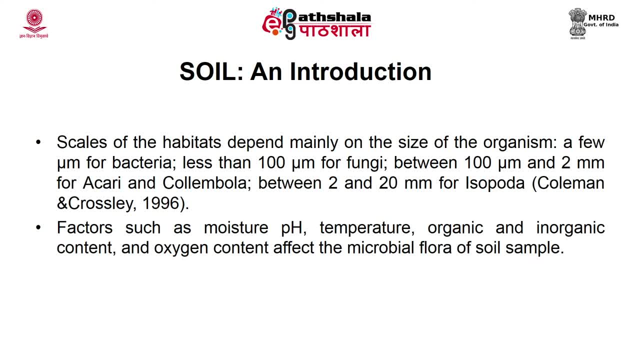 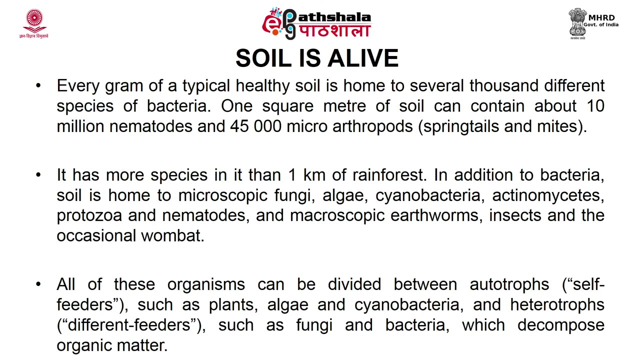 beneath the surface of the soil. the soil environment differs from one location to another and also from season to season. therefore, factors such as moisture, ph, temperature, organic and inorganic content, as well as the oxygen content, affects the microbial flora of the soil samples. every gram of a typical healthy soil is the home for several hundred. 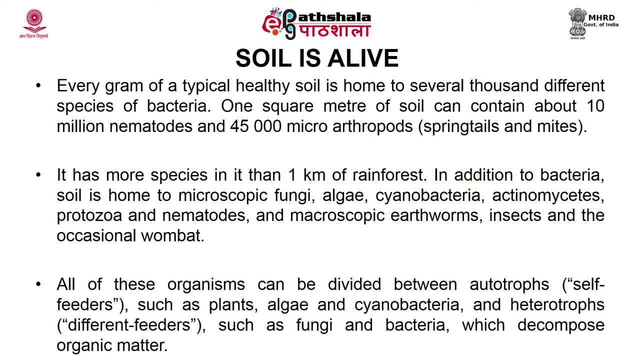 to several thousand different species of bacteria. in addition, soil is also home to microscopic fungi, algae, cyanobacteria, actinomycetes, protozoa, nematodes and macroscopic earthworms and insects. all these organisms can be divided between autotrophs, which are these self feeders such as 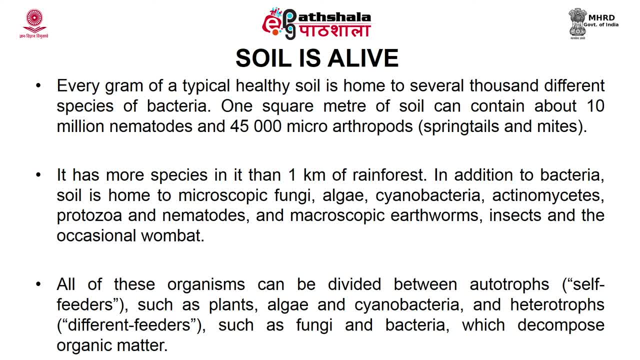 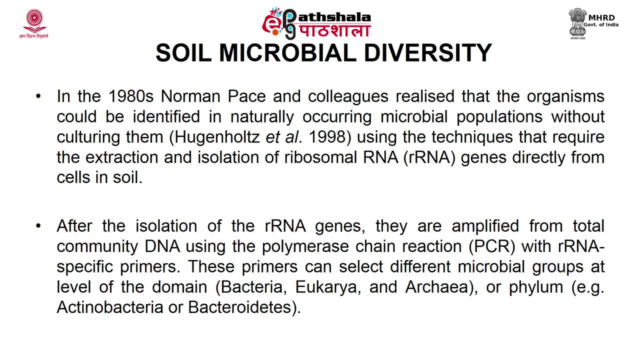 plants, algae and cyanobacteria, and the same thing can be used to supplement the soil from organic or Second category is heterotrophs, which are different feeders like fungi and bacteria which decompose the organic matter. The studies of soil microbial diversity has revealed that only less than 10 percent of 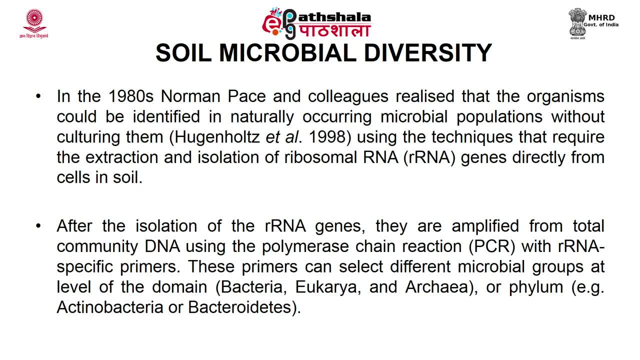 the soil microbial community could be readily cultured. So 90 percent of the non-culturable microorganisms could be identified in their naturally occurring microbial population without culturing them in the lab conditions For this. the techniques they are used: they include extraction and isolation of ribosomal 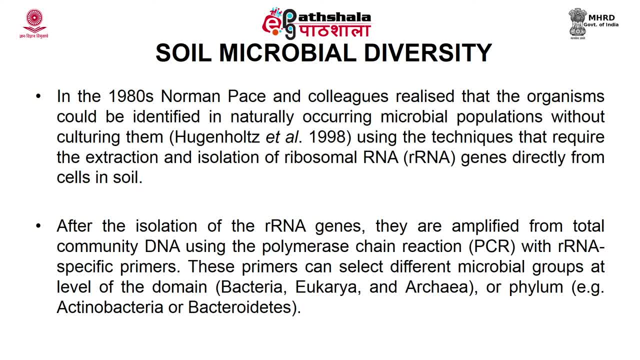 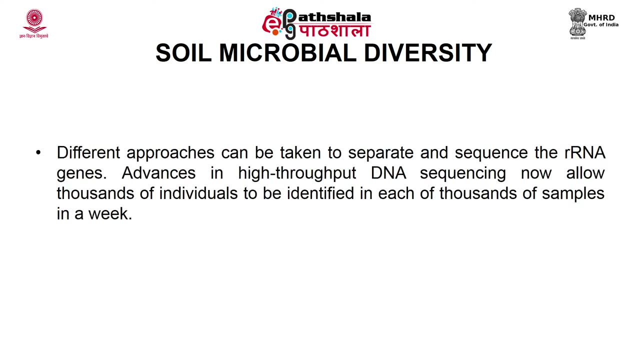 RNA genes directly from the microbial cells which are present in the soil. After the isolation of ribosomal RNA genes, they are amplified from the total community DNA using the PCR with rRNA specific primers of that community. Thank you. These primers can select different microbial groups at the level of a domain and different. 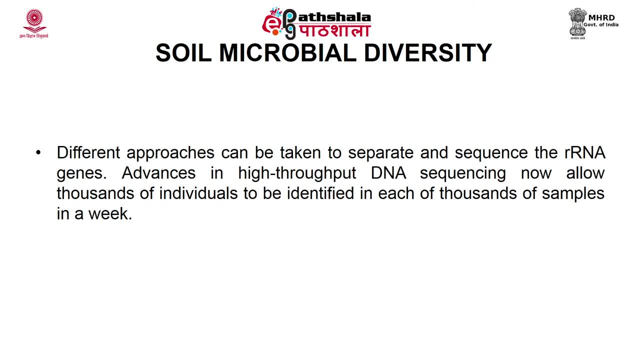 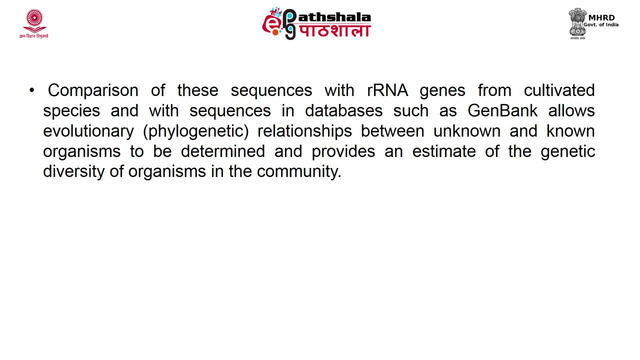 approaches can be taken to separate and sequence the rRNA genes, and this will finally contribute for the microbial diversity analysis By comparing the sequences of the rRNA genes from the cultivated species and the sequences which are already present in the databases, such as NCBI's gene bank. 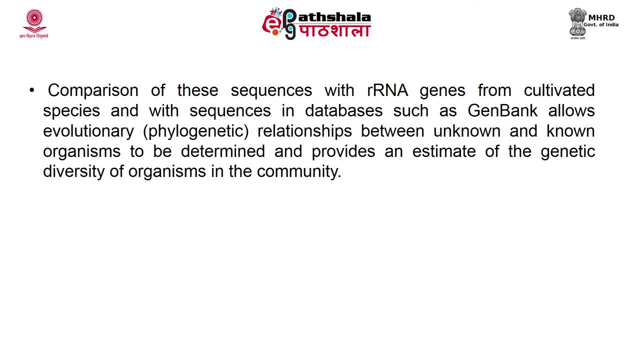 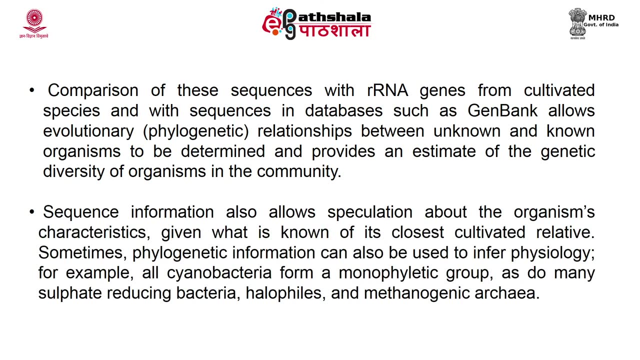 The phylogenetic relationship between the unknown and the known organisms are determined, and it provides an estimate of the genetic diversity of the organisms which are present as a community. The sequence information also allows the organism's characteristics, given what is known of its closest cultivated relative. 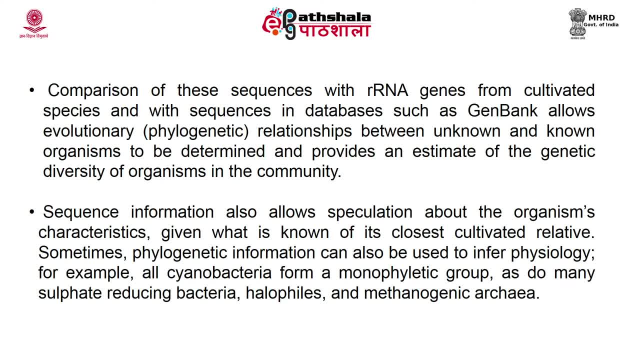 Sometimes this phylogenetic information can also be used to determine the genetic diversity of the organisms In furphysiology, for example, all cyanobacteria. they form a single monophyletic group, as do many sulfur reducing bacteria halophiles and methanogenic archaeobacteria. 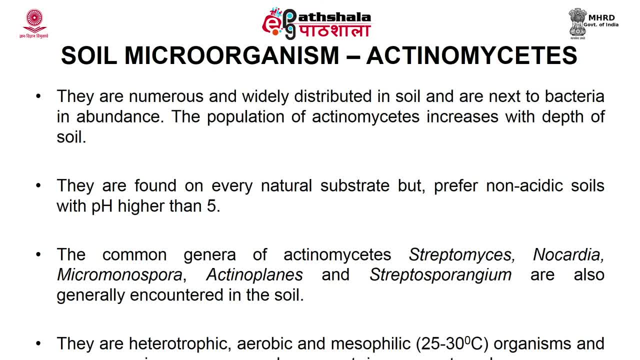 Now, as we had talked about the kind of soil microorganisms, now let's start the study of these microorganisms one by one. First, soil microorganisms: actinomycetes. Actinomycetes are numerous microorganisms. Actinomycetes are numerous microorganisms. 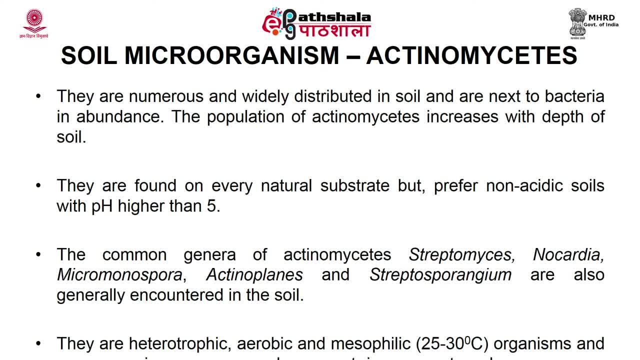 Actinomycetes are numerous microorganisms. Actinomycetes are numerous and widely distributed in the soil, and they are next to bacteria in their abundance. The common genera of actinomycetes are streptomycetes, which corresponds to roughly 70% of the total. 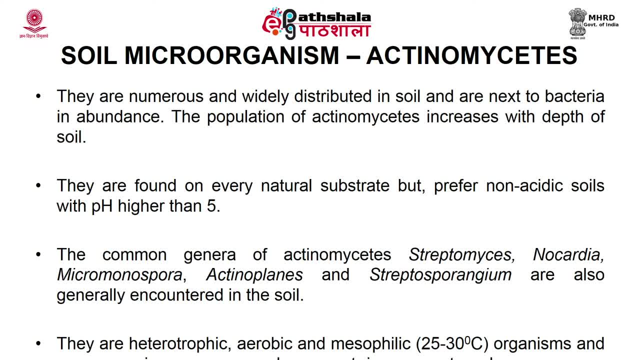 actinomycete population present in the soil. nocardia, micromonospora and streptosporangium are also generally encountered in the soil. Actinomycetes are widely distributed in the soil as well as in the compost and the population. 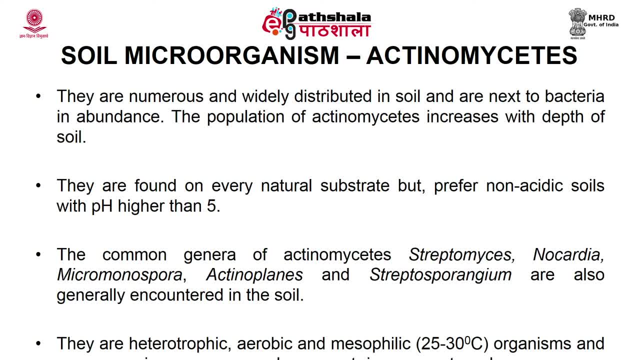 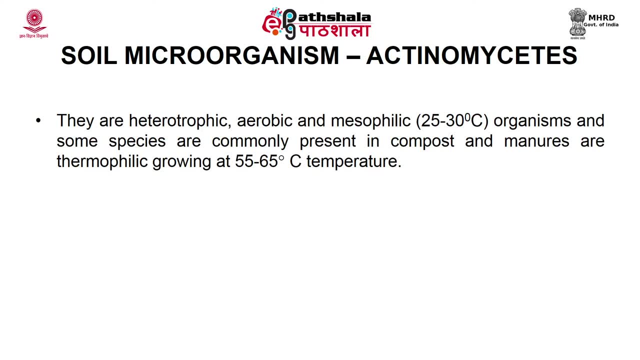 of these actinomycetes. it increases with the depth in the soil. They are found on every natural substrate, but they prefer non-acidic soils which are having the pH range higher than 5.. They are heterotrophic, aerobic and mesophilic, means they love to grow at the temperature. 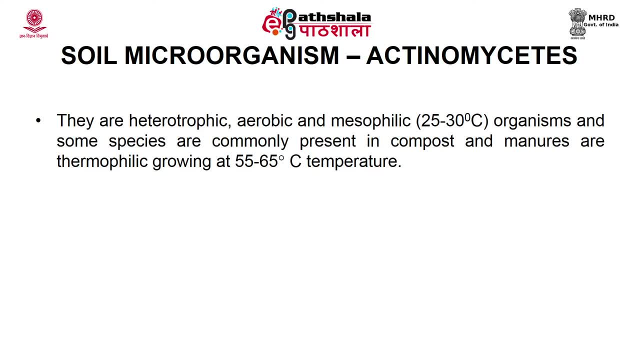 of 25 to 30 degree Celsius, And some species which are commonly present in the soil are called the mesophilic. They are also known as mesophilic and mesophilic, While most of the bacteria they are found in the top foot or the top soil: the actinomycetes. 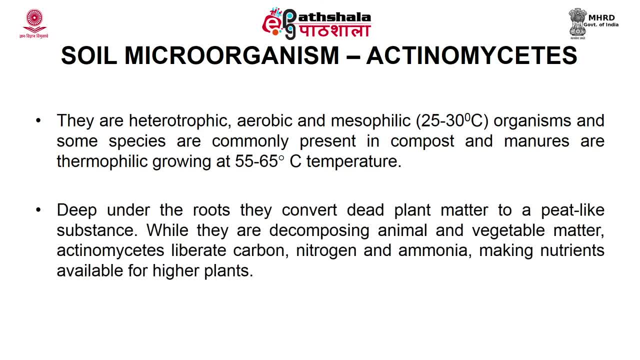 work many feet below the surface. Deep under the roots, they convert the dead plant matter to the organic substances. While they are decomposing animal and vegetable matter, they also liberate carbohydrates, minerals and minerals- They are also known as carbon nitrogen, ammonia- and thus making the nutrients available. 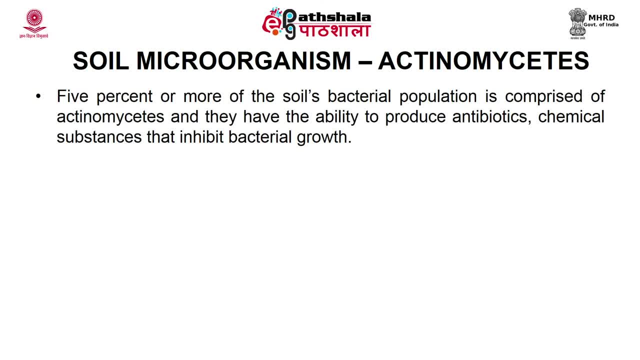 for higher plants. 5% or more of the soil microbial population is comprised of actinomycetes, and they are having the ability to produce antibiotics also. Antibiotics are the chemical substances that inhibit the bacterial growth, and these are the organisms with characteristics common to both the bacteria and the microorganisms. 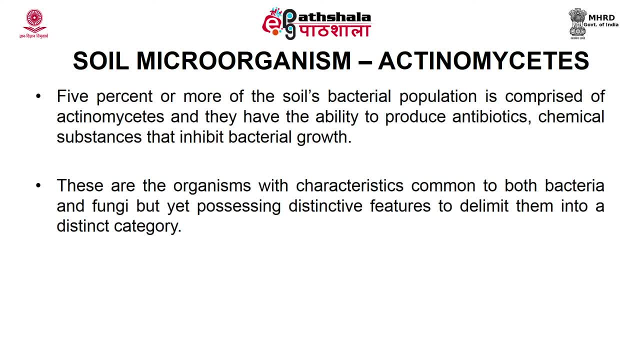 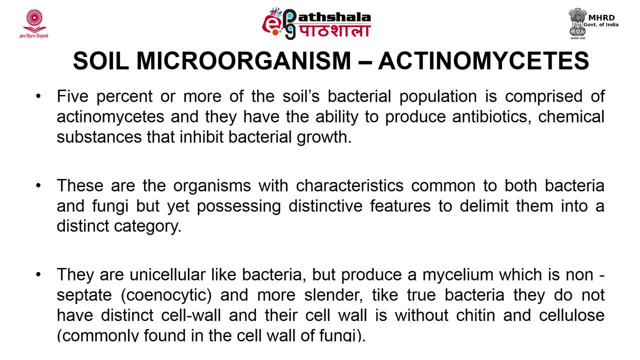 But yet they possess the distinctive features These actinomycetes. they are unicellular, like the bacteria, but produce a mycelium which is non septate- This condition is also called synocytic- and the mycelium is more cylinder. 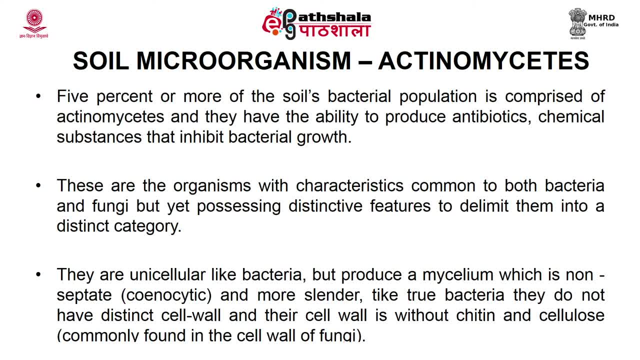 Like the true bacteria, they do not have distinct cell wall and their cell wall is without chitin and cellulose. And the chitin and cellulose they are commonly found in the cell wall of fungi, On the culture media, the slimy distinct colonies of crew bacteria which grow very quickly. 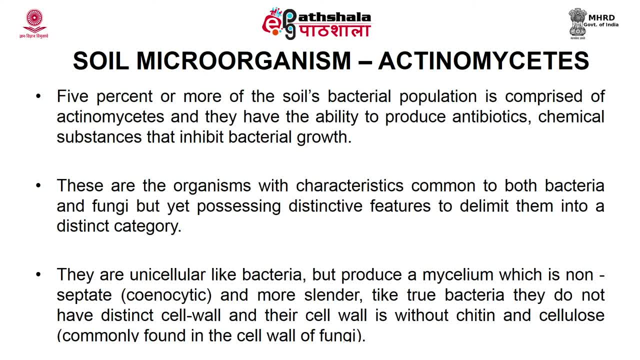 But the actinomycetes colonies. they grow slowly and they show the powdery consistency and they stick firmly to the agar surface. They produce the hyphae and conidia. like the fungi, Certain actinomycetes also have the segmented hyphae, which resemble bacteria both morphologically and physiologically. 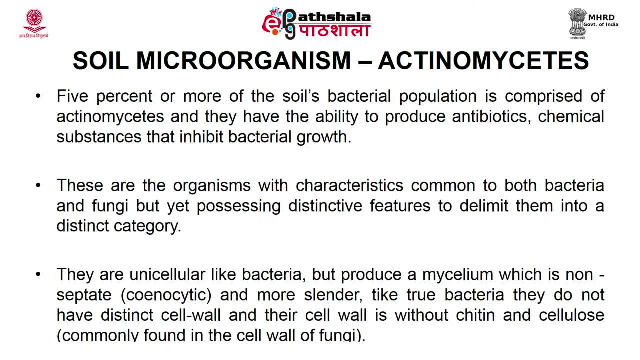 So we can say that these actinomycetes they are having some of the characters like bacteria and some of the characters resemble the fungi, But still it's a distinct category. The characteristic earthy smell of the newly plowed soil in the spring season is caused by these actinomycetes. 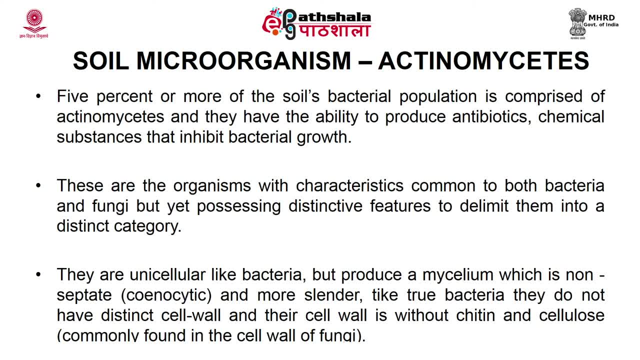 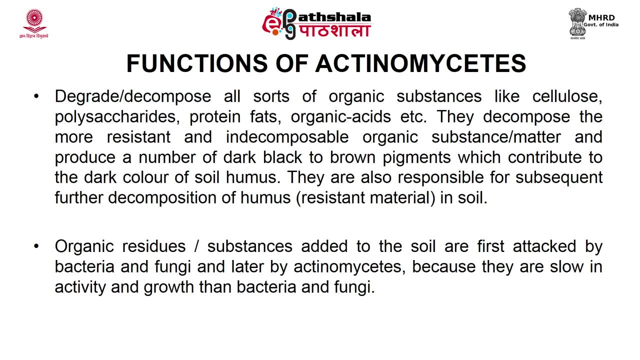 A higher form of bacteria which is similar to fungi and molds, And these actinomycetes. they are especially important in the formation of the humus by slowly breaking down the humic acid which is present in the soil. Now let's discuss the functions of actinomycetes. 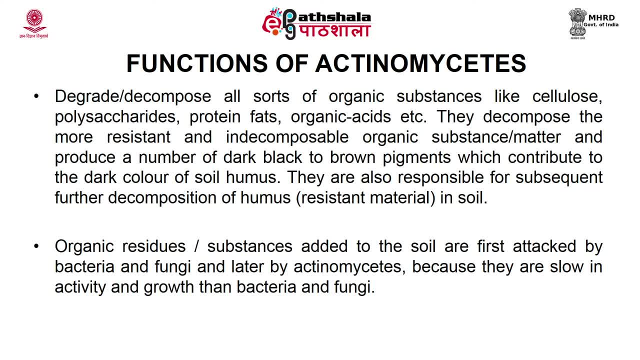 As I have already discussed that, these actinomycetes. they decompose all sorts of organic substances like cellulose polysaccharide, Proteins, fats and organic acids, So they are very good decomposers. The organic residues and the substances which are added to the soil are first attacked by bacteria and fungi. 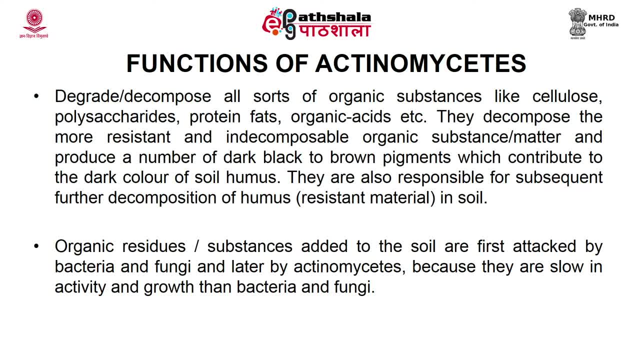 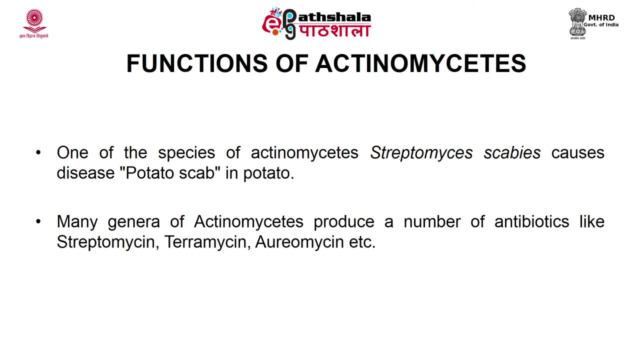 And later on, the actinomycetes. they attack on this semi-hydrolyzed organic residues because they are slow in activity as well as their growth is also slow as compared to bacteria and fungi. These actinomycetes, they decompose the more resistant and the indecomposable organic substance and produce a number of dark, black to brown pigments which contribute to the dark color of soil: humus. 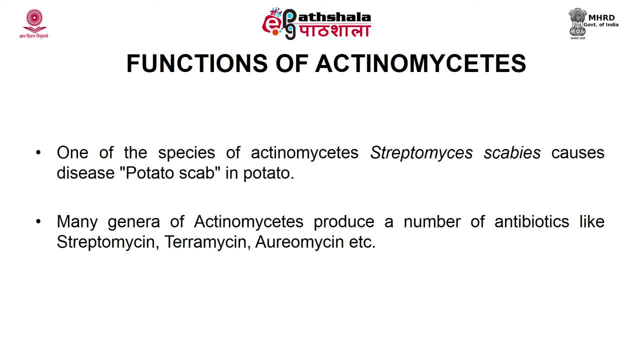 They are also responsible for the subsequent further decomposition of the humus in the soil. These actinomycetes are also responsible for the earthy smell of the freshly plowed soil. Many genera of the actinomycetes. they synthesize a number of antibiotics like streptomycin, teramycin, oreomycin. 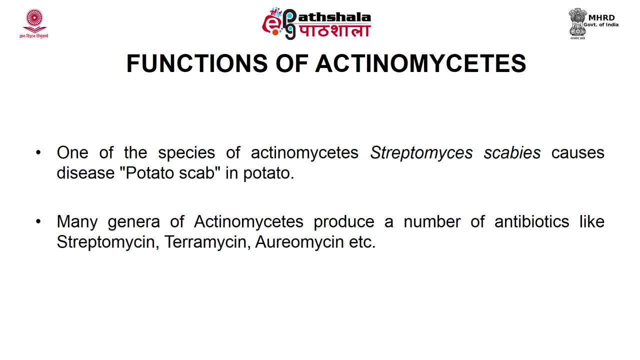 All these antibiotics. they are secreted by the actinomycete streptomyces species. One of the actinomycete species is also causing the disease, Namely streptomycete scabies. which is causing the disease: Potato scabies. 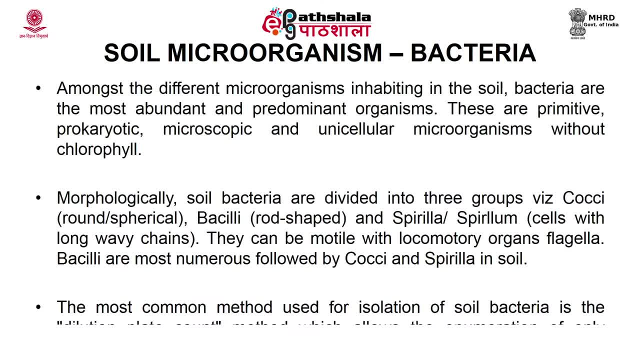 Potato scab in the potato crop. Now, after actinomycetes, let's start with soil bacteria. Bacteria are the smallest single celled microorganisms, which are having the shape either a cocus, a rod or a spiral twist, And they are most abundantly found in the soil. 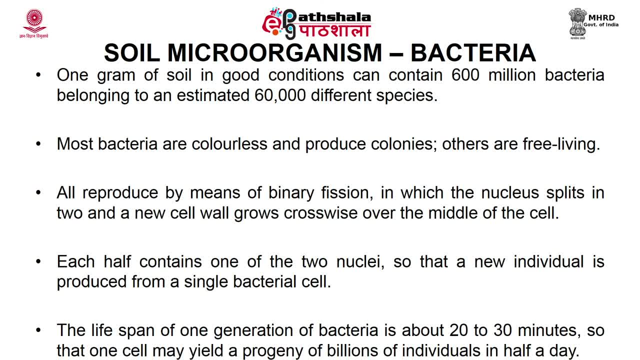 One gram of the soil in good condition can contain 600 million bacteria Belonging to an estimated 60,000 different species, Most of which have yet to be even named, And each is having its own role and capabilities. Most bacteria are colorless and produce colonies. 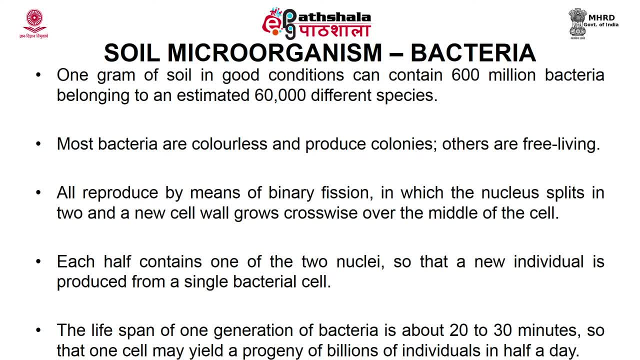 Others are free living, All of them. they reproduce by means of binary fission, In which the nucleus splits into two And the new cell wall grows crosswise Over the middle of the cell. So each half of the cell contains one of the two nuclei. 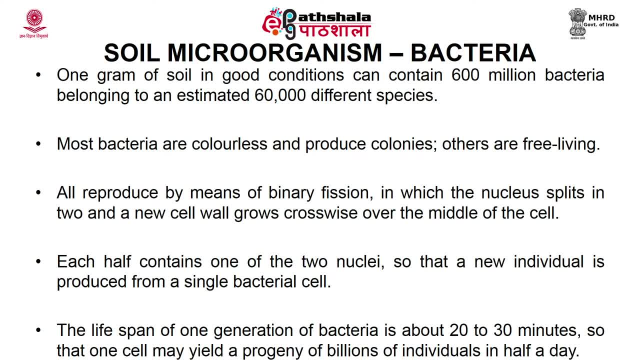 And the new individual produced from the single bacterial cell is having the same nuclear composition. Under the best conditions, a colony of bacteria can multiply into billions in a very short time span, And the time span for one generation of bacteria is about 20 to 30 minutes. 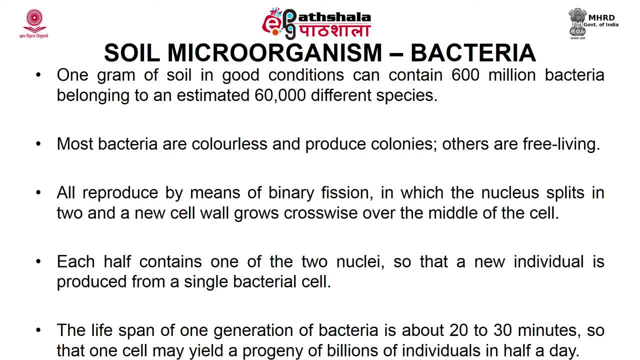 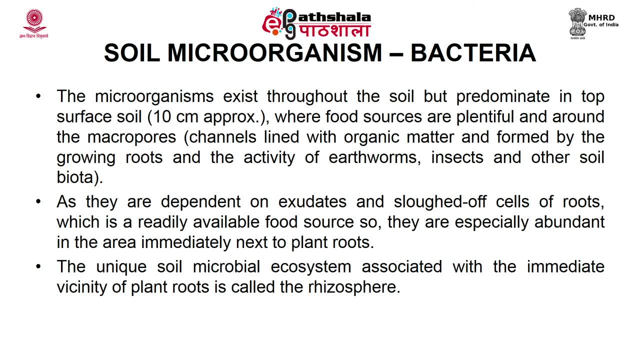 So it means The cells may yield progeny or billions of individuals in just half of a day. The microorganisms exist throughout the soil, But they predominate in the top surface soil. In the top surface soil, the food sources are plentiful. 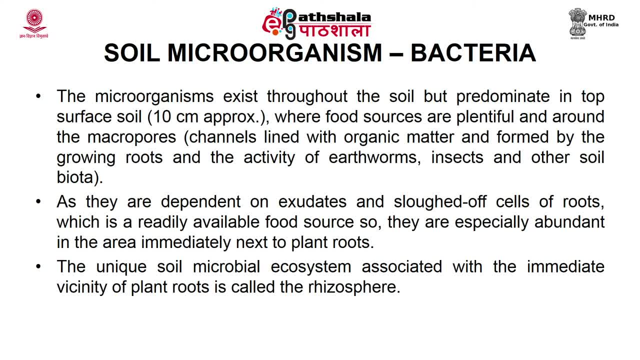 And they are also present around the macropores, As they are dependent on the root exudates and the slugged off cells of the root, Which is a readily available food source for these bacteria. That's why they are abundant in the area immediately next to the plant roots. 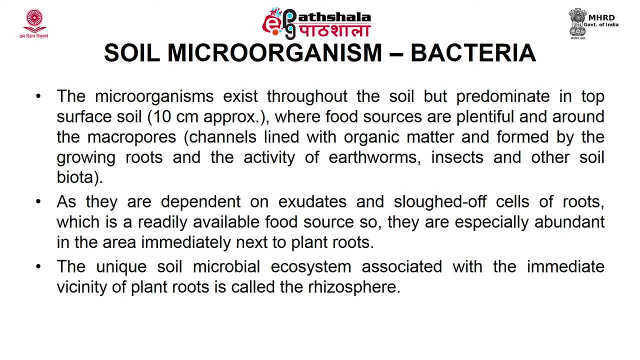 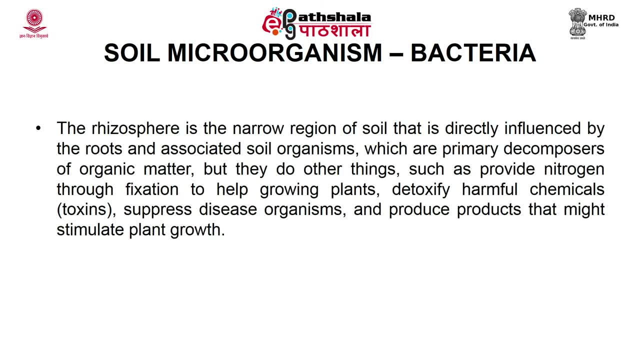 The unique soil microbial ecosystem Associated with immediate vicinity of the plant roots Is called the rhizosphere. The rhizosphere is the narrow region of the soil That is directly influenced by the root And the associated soil organism, Which are primarily the decomposers of the organic matter. 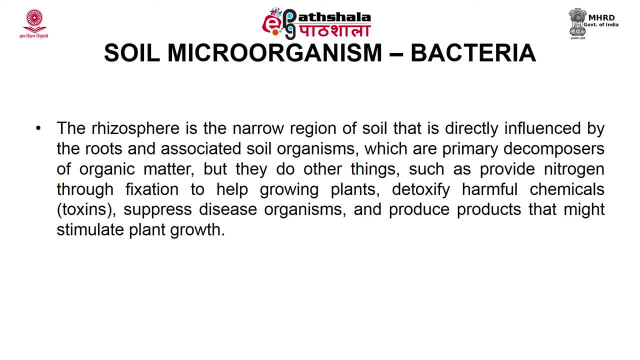 Among the different microorganisms Inhabiting in the soil, Bacteria are most abundant And predominant microorganism. They are primitive, Prokaryotic, Microscopic And unicellular microorganisms, Without chlorophyll Bacteria being the prokaryote. 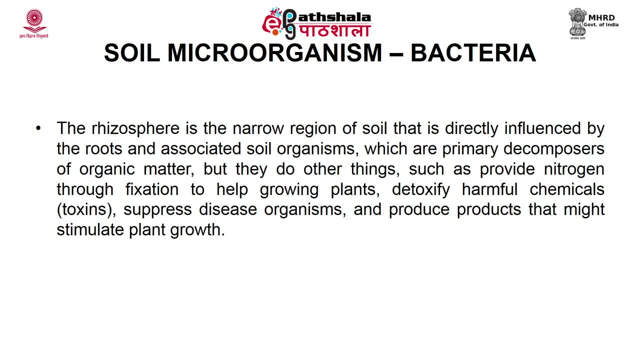 Does not possess well defined nucleus, And the single chromosome Which is present in a bacterial cell Consists of a double hallux DNA Lying naked in the cytoplasm. This double hallux DNA Is attached to the membrane folding 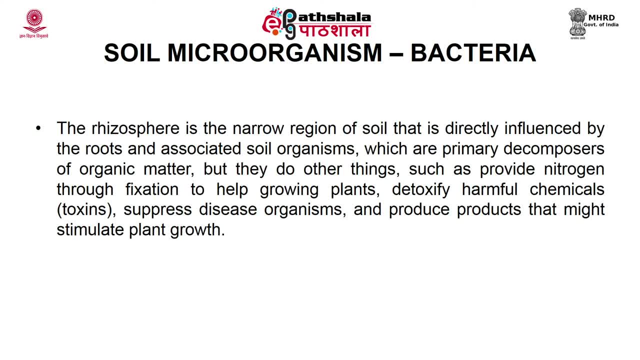 Which is called mesosome. The only cell organelle Which is present in the bacterial cell Is the ribosomes, Which are of 70S type. This bacterial cell Is enveloped by the cell wall, Which is a tough, rigid structure. 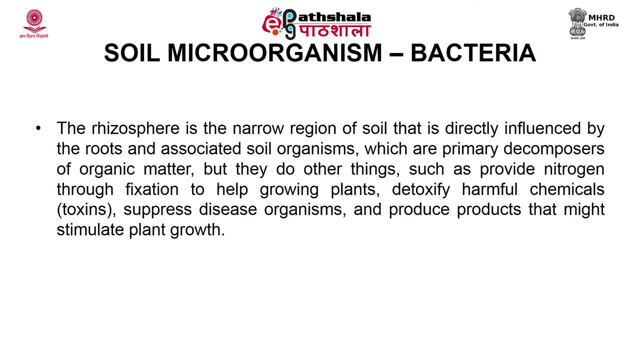 Made up of peptidoglycan, Lipopolysaccharides And techoic acid. Some bacteria Do have a jelly like outer covering That surrounds the cell wall And this jelly like Covering is called capsule. 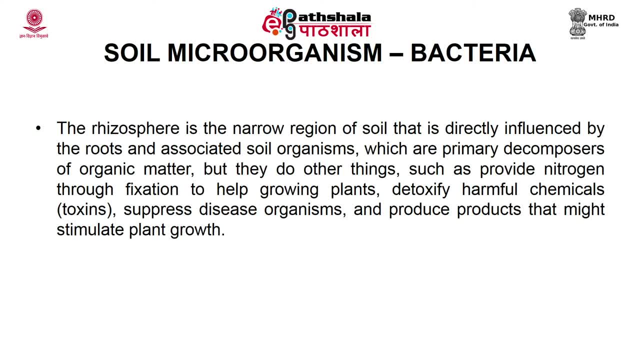 This capsule Is either consisted of Polysaccharides And occasionally of polypeptide And hyaluronic acid. Sometimes The short filaments Are extruding from the cytoplasmic membrane And they are called. 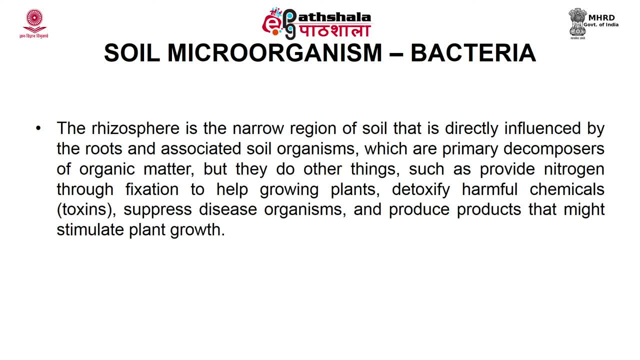 Fimbri or pili. Based upon the morphological Features of bacteria, They are classified as gram positive Or gram negative Based upon the staining method Given by Danish physician Hans Christian. Gram Gram has given staining method In which, based upon the 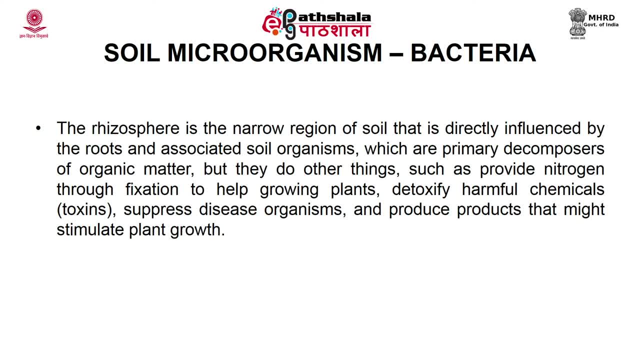 Lipopolysaccharide, content Of the different Present in the cell wall of the different bacteria, Either the bacteria. They will have the violet color Or they will have the pink color In this gram staining process. The gram positive bacteria. 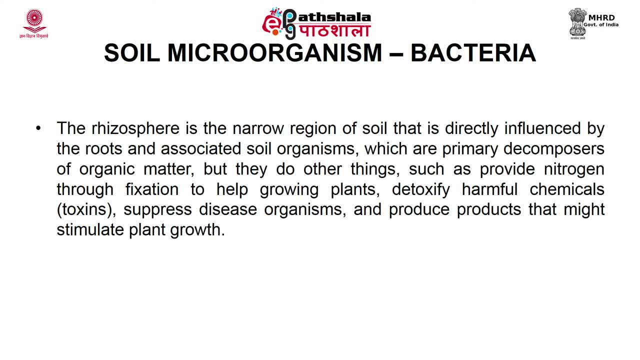 They will have the purple color, The violet color and the gram negative bacteria. They will have the pink color. The most common method For isolation of soil bacteria Is the dilution plate count method, Which allows Only viable cells To grow. 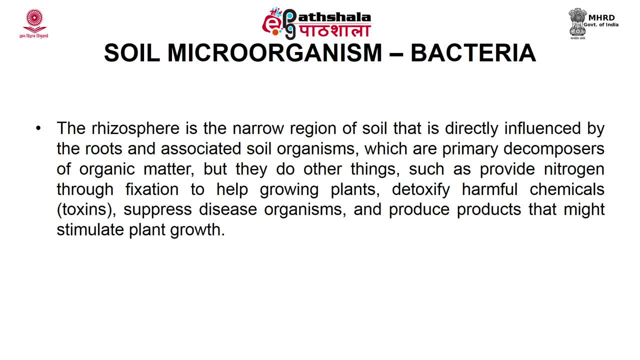 On the basis of ecological Characteristics, Other microorganisms Are classified into two broad categories: Autotonous As well as Zymogenous. Autotonous bacterial population Is uniform and constant in the soil Because Their nutrients they are derived. 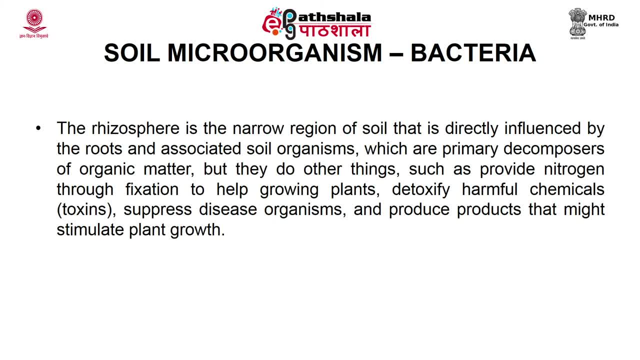 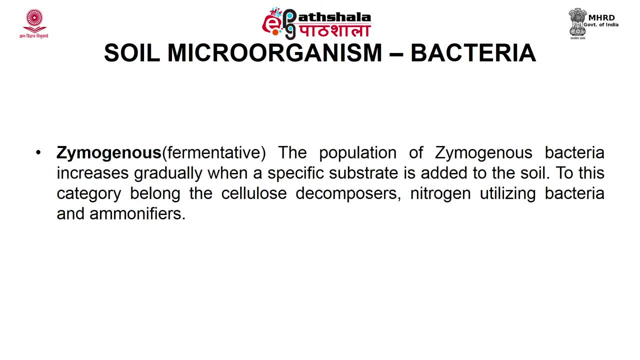 From the native soil organic matter- Example Arthrobacter and nocardia- Whereas the second category, Zymogenous bacterial population In the soil- is low, As they require An external source of energy And the presence of this. 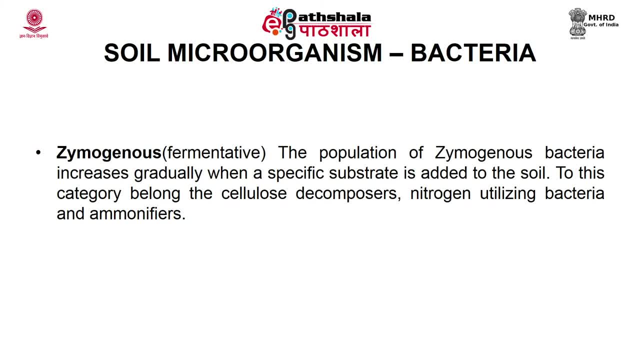 Zymogenous bacteria Increases gradually When a specific substrate is added to the soil. Example: Cellulose decomposes Nitrogen utilizing bacteria And ammonia fires. They belong to this Zymogenous category- Zymogenous bacteria. They are not the native. 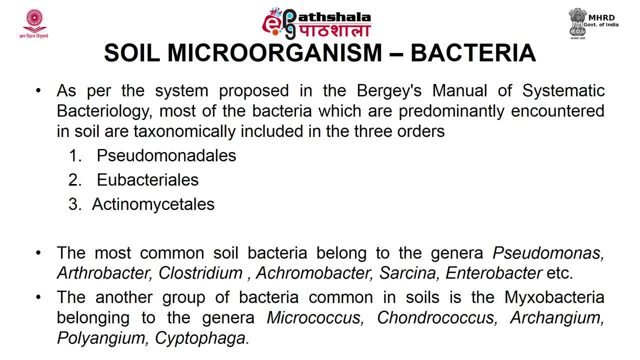 Population of the soil. In the system proposed in the Burge's manual of systematic bacteriology, Most of the bacteria Which are predominantly Encountered in the soil. They are taxonomically included In the genera Pseudomonas. 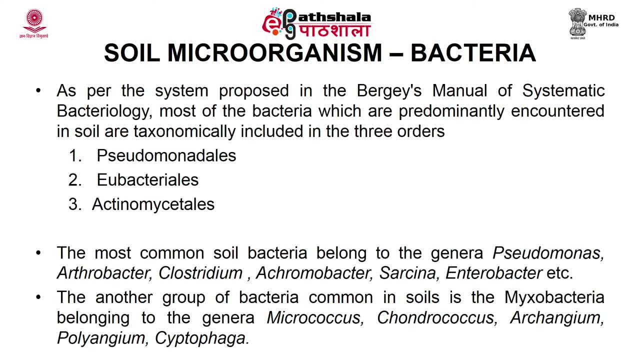 Arthrobacter Clostridium, Achromobacter And enterobacter, The another group of bacteria Which is common in the soil: Chondrococus, Arachangium, Polyangium And septophaga. 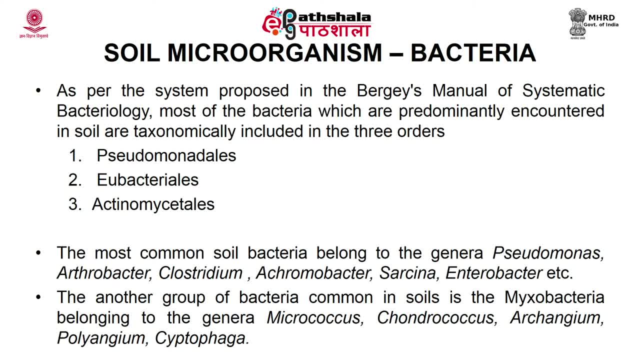 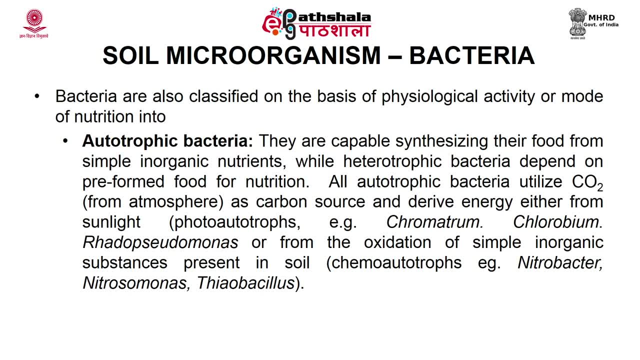 On the basis of physiological activity, The bacteria, they are classified Into two categories: Autotrophic bacteria And heterotrophic bacteria. Autotrophic bacteria: They are capable of synthesizing their food From simple inorganic nutrients, While Heterotrophic bacteria- 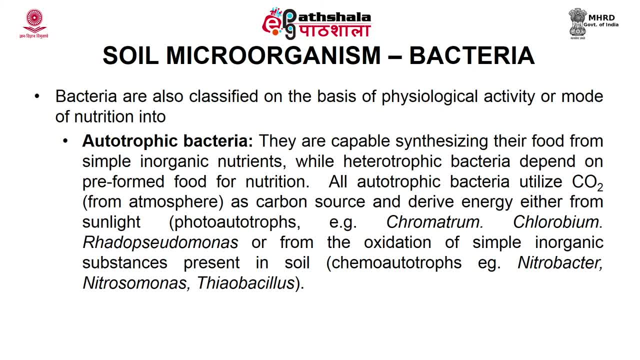 They depend upon Food for nutrition. All autotrophic bacteria Utilize carbon dioxide Present in the atmosphere As the carbon source And derive the energy Either from sunlight Or from the oxidation of simple Inorganic substances Present in the soil. 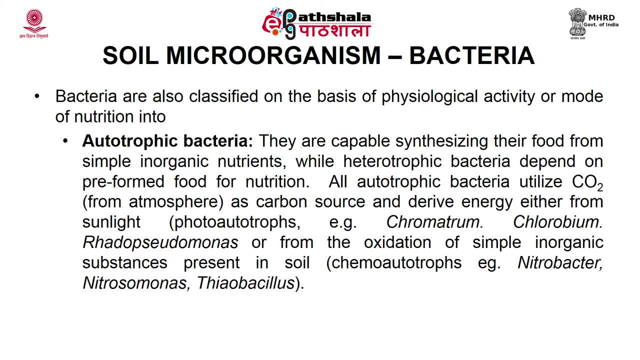 The former category belongs to phototrophs And the later category Belongs to chemotrophs. The common example Of phototrophs are Chromatrum, Chlorobium And rhodosedomonas, And the example of chemotrophs is: 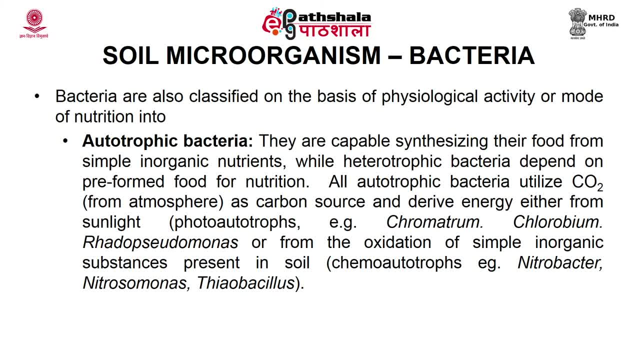 Nitrobacter, Nitrosomonas And thiobacillus, Moving ahead To heterotrophic bacteria. Majority of the soil bacteria Are heterotrophic in nature, As they derive their carbon and energy From complex organic substances Present in the soil. 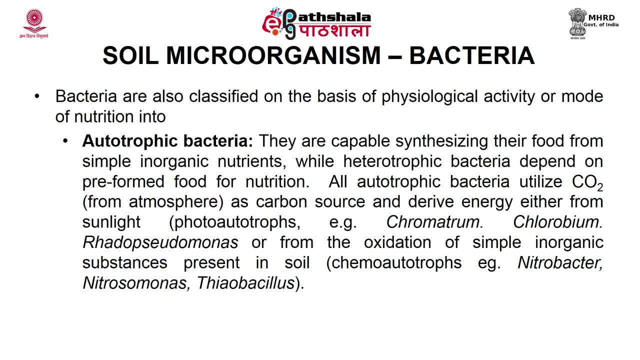 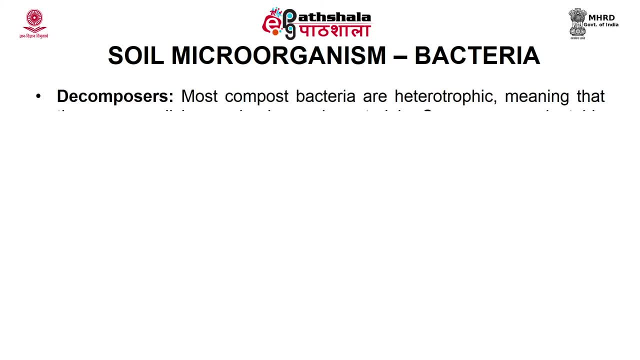 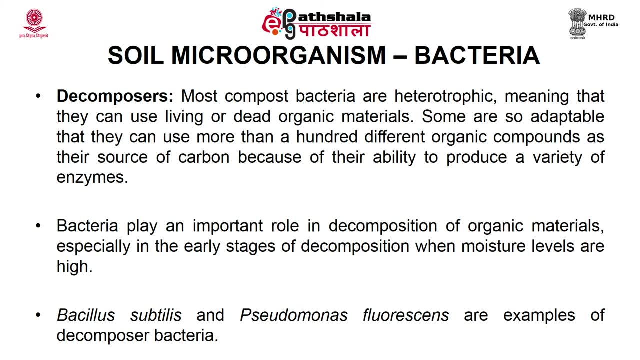 Certain bacteria Also require Specific amino acids, Vitamins And other growth promoting substances For their growth. Another class of bacteria Belongs to decomposers. These bacteria are smaller, Less mobile, Less complex Than most of the organisms. 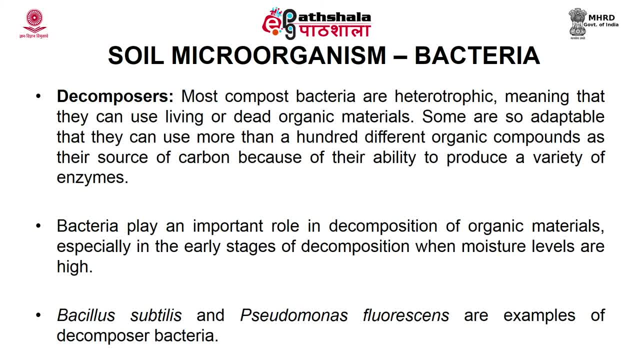 Therefore, they are less able to escape An environment that becomes unfavorable. Bacteria Are most nutritionally diverse Among all the categories of organisms, Which is to say As a group They can be eat nearly anything. Most compost bacteria Are heterotrophic. 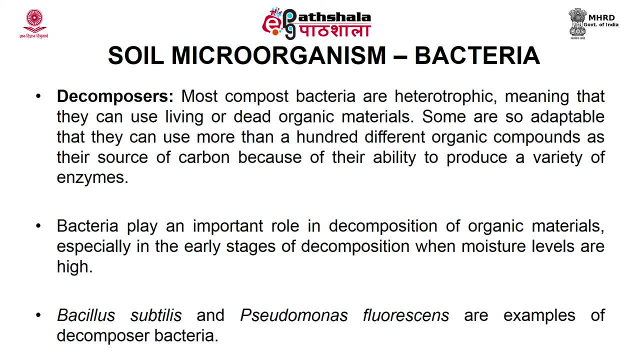 That is, they can use Either living or dead organic material. Some are so adaptable That they can use more than a hundred Different organic compounds As their source of carbon Because of their ability to produce A variety of enzymes. Usually they can produce 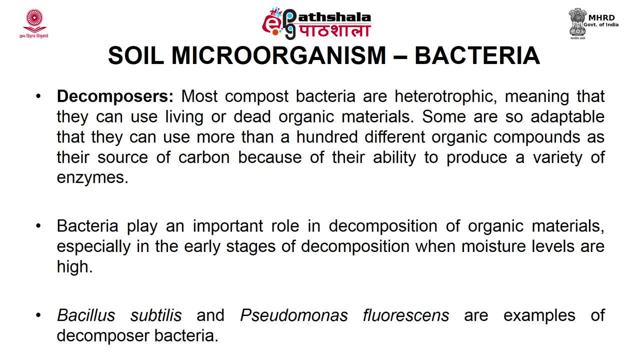 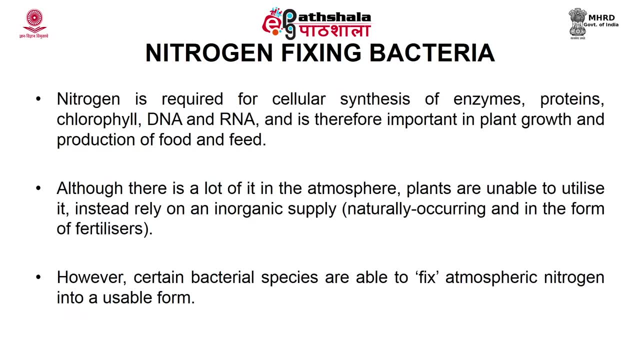 The appropriate enzyme To digest whatever the material They find for themselves. In addition, The respiratory enzymes In the cell membrane Make aerobic respiration possible As an energy source For the compost bacteria. Another very distinctive class Of bacteria are: 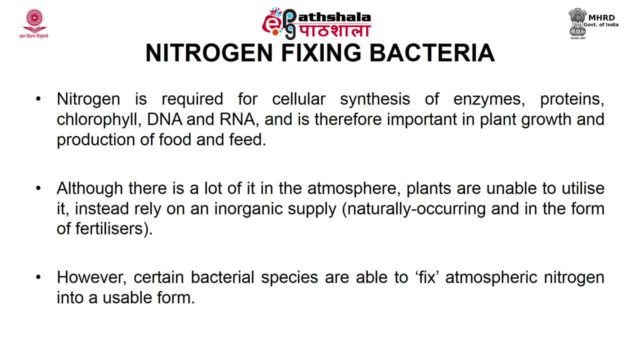 Nitrogen fixing bacteria. We all know that nitrogen is required For cellular synthesis And for the production of Proteins- proteins, chlorophyll, DNA, RNA- And therefore it is very important In plant growth and production. The ability of crop plant. 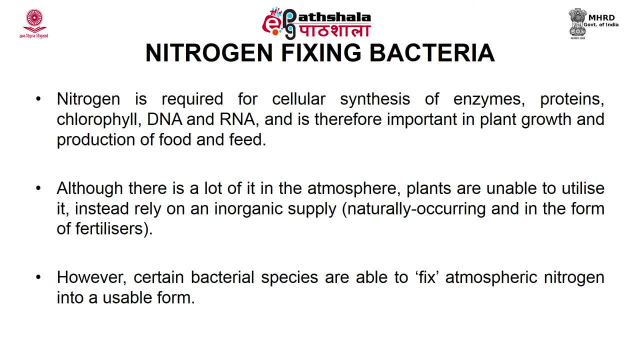 To thrive is frequently limited By the supply of available nitrogen, Although there is a lot In the atmosphere, But the plants are unable to utilize it. Instead, They rely on the inorganic supply Which is available to them In the form of fertilizers. 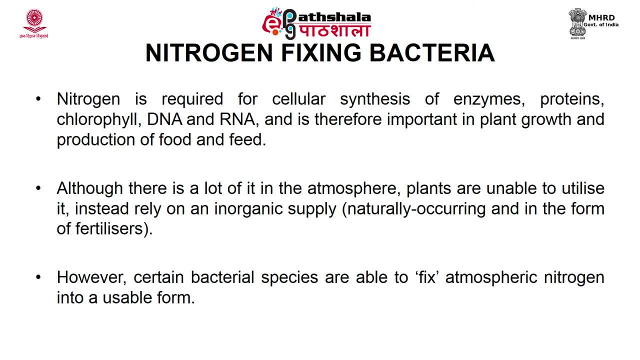 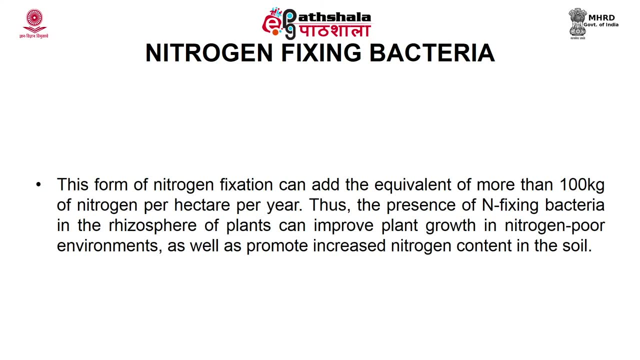 But certain species of bacteria. They are having the capacity To fix the atmospheric nitrogen Into the usable form, Ammonia, As well as the nitrites and nitrates, Which are readily utilized By the plants. This phenomenon of nitrogen fixation- 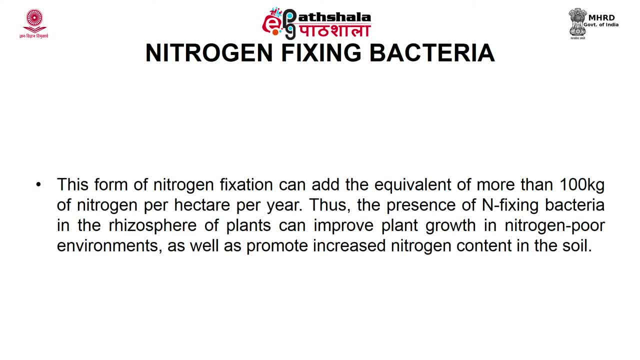 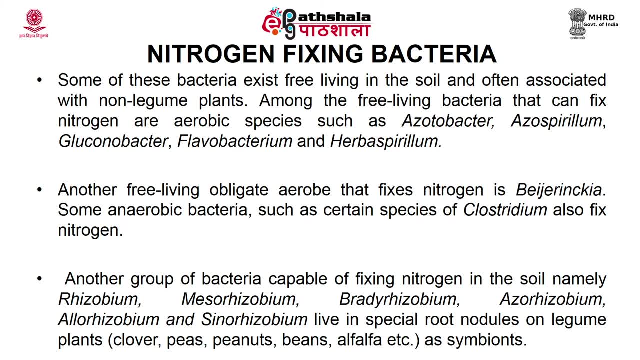 Can add more than 100 kg Of nitrogen per hectare Per year. Some of the bacteria Which belong to this nitrogen fixers. They exist For free, living in the soil, Or they are associated With the roots of the non-legume plants. 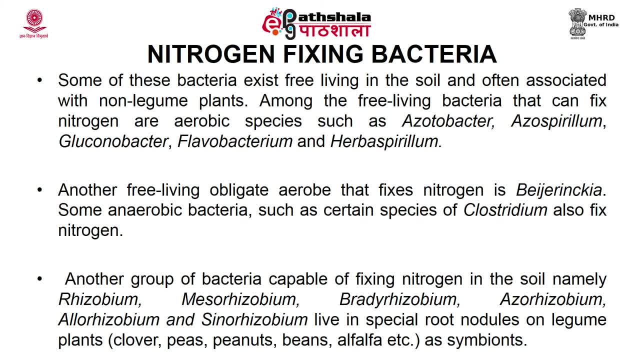 The free living bacteria Present in the soil That can fix the nitrogen Are aerobic species, Which belong to Azotobacter, Azospirulum, Gluconobacter, Flavobacterium And herbospirulum. 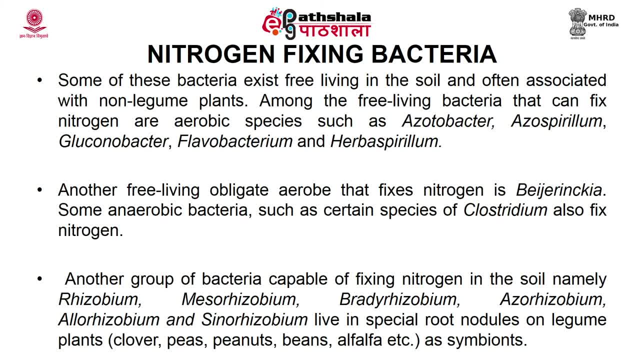 These aerobic organisms. They shield the Nitrogen into ammonical nitrogen From the oxygen, As they are having A very high rate of oxygen use, So in this way They minimize the diffusion of oxygen Into the interior of the cell. 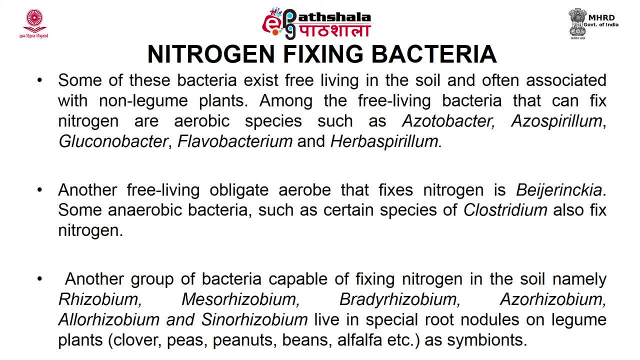 Where the enzyme is Located. The free living obligate aerob That fixes nitrogen Is baserenchia And the anaerobic bacteria. They are also Fixing the atmospheric nitrogen And they belong to The genus Clostridium. 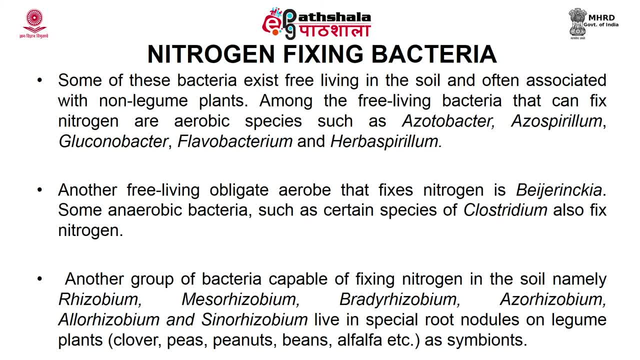 Another group of bacteria Which are capable of fixing nitrogen In the soil, Like rhizobium, Mesrhizobium, Breddyrhizobium, Ezrhizobium, Ellorhizobium And sinrhizobium. 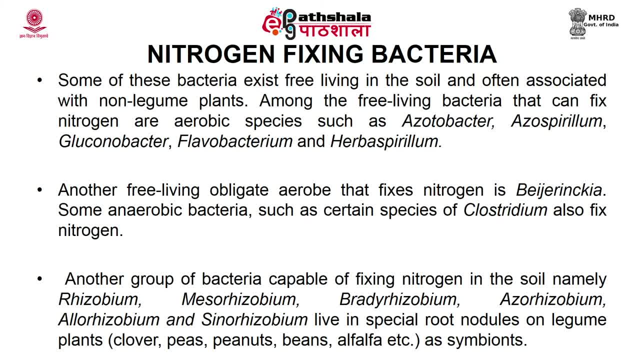 They live in the root nodules Of the leguminous plants, Like clover, Pea, As the symbionts, The free living rhizobium Which is present In the plant root After the infection of the root. 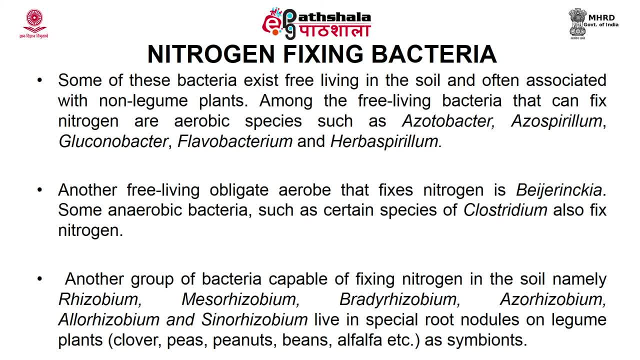 It infect the root cells. Normally it forms Rod shaped cells Which proliferate And it will lead to the formation Of the root nodules in the leguminous plants. You can see A nodulated root of the legume plant. 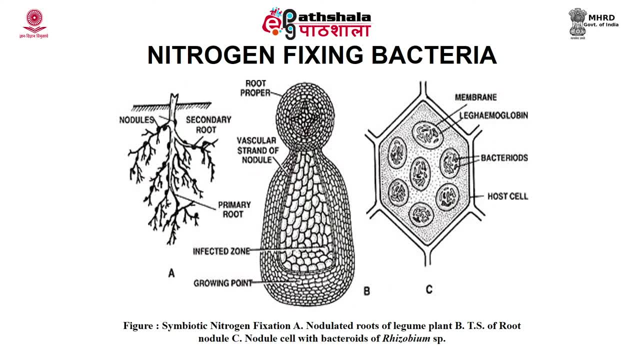 And the bacteroid structure Of the root nodules In the slide. There are so many examples Of symbiotic nitrogen fixation In the non leguminous plants also, Such as trees. The elder tree Is symbiotically infected. 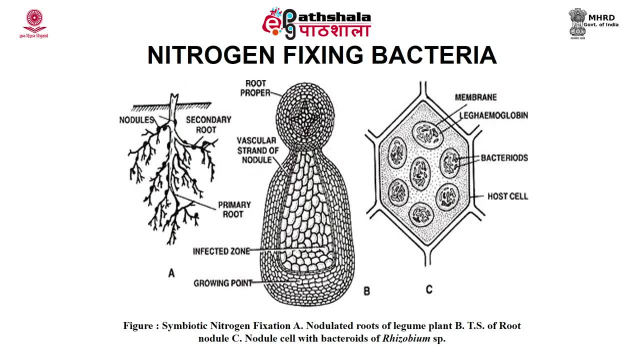 With the actinomycete And forms the nitrogen fixing Root nodules. Nitrogen fixing bacteria Belong to different phyla Of the domain eubacteria And they are present In the roots of the plants In more or less specific manner. 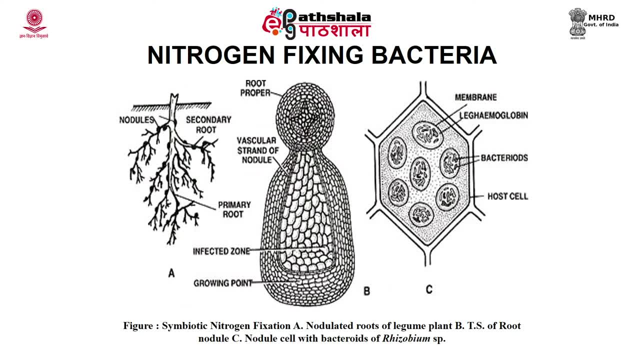 In the roots. They are leading to the formation Of the root nodules And they have higher activity In relation to the host. However, some bacteria May inhabit the root surface Or the plant rhizosphere, Forming associations With low degree of specificity. 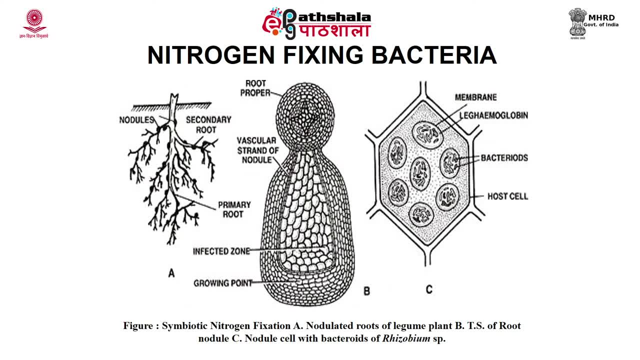 With the host Plants associated with these bacteria Benefit themselves Due to increased Nitrogen supply And, in the case of symbiotic association, Over 90 percent Of the nitrogen Contained in the plant Can be fixed by bacteria. 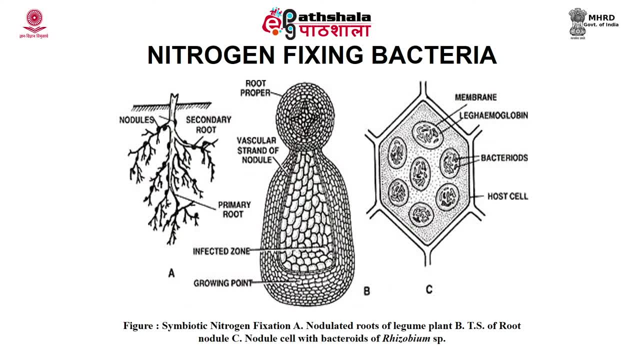 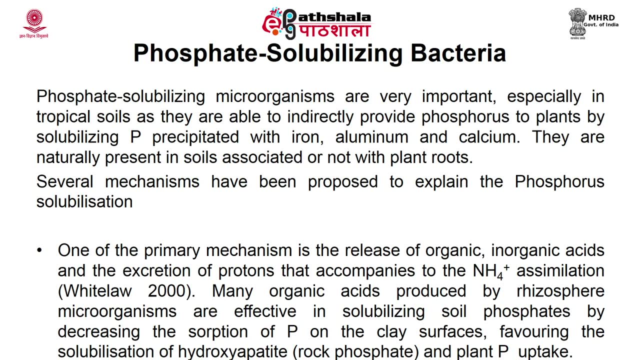 Thus, the presence of nitrogen fixing bacteria In the rhizosphere of the plant Can improve the plant growth In nitrogen poor environments, As well as promote Increased nitrogen content Of the soil. Another class of bacteria. It belongs to phosphate. 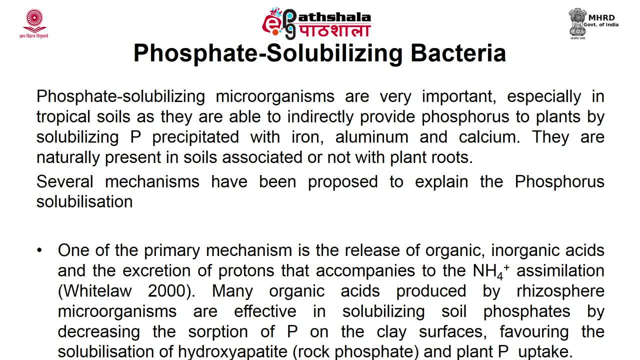 Solubilizing microorganisms. Another category of the microorganism Present in the soil Belongs to phosphate Solubilizing microorganism. These microorganisms Are naturally present in the soil And they are also associated With the plant roots. 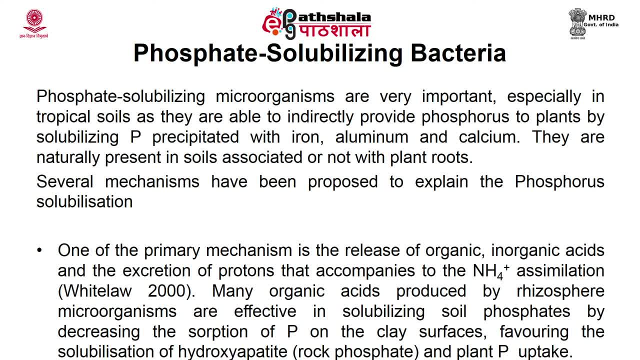 Or they are present in the rhizosphere area. These phosphate solubilizing microorganisms Are very important In the tropical soils As they are able to Indirectly provide Phosphorus to the plants By solubilizing the total phosphorus. 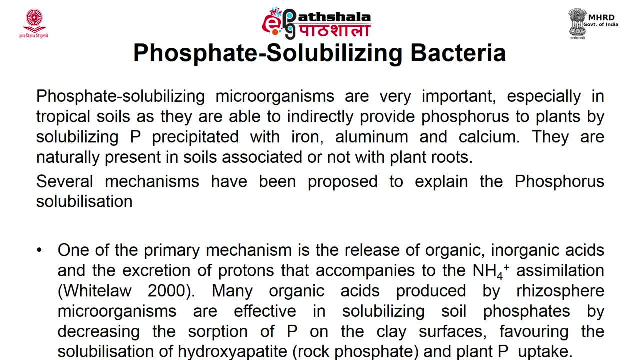 Present in the soil, Associated with Iron, aluminium And calcium. These microorganisms Solubilize the phosphorus Adsorbed by soil minerals By means of various mechanisms, And these mechanisms They are shown on the slide. 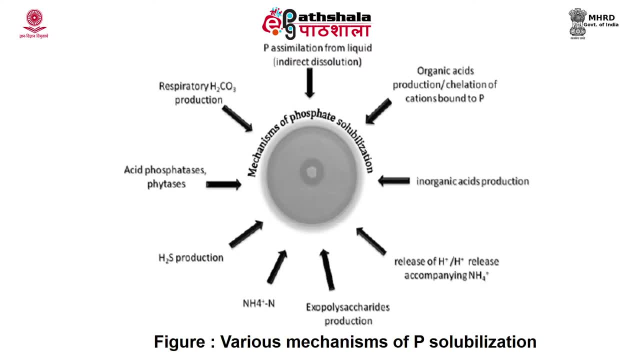 These mechanisms which have been proposed To explain the phosphorus solubilization Are The release of organic Or inorganic acids, Excretion of protons Which accompanies the Ammonia assimilation, So the release of these organic. 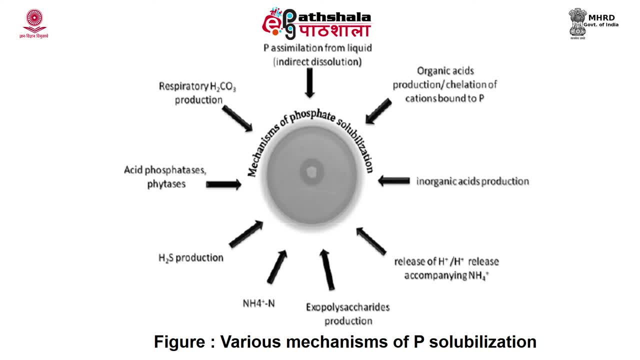 And inorganic acids Into the soil Will decrease the pH of the soil In the localized area And will make the precipitated phosphorus To get dissociated And then it becomes available To the plant. Many organic acids In the plant. 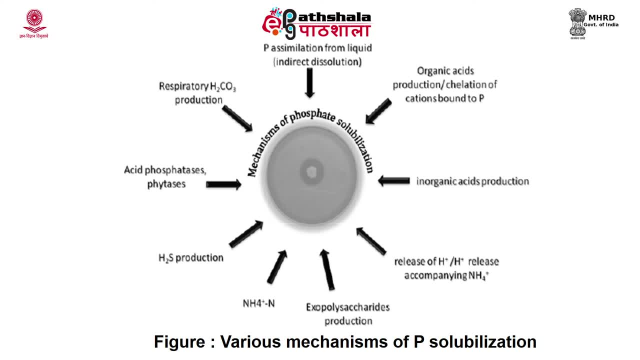 But in the home, As you can see, The phosphorus Is produced by The phosphorus In the soil, So so There is a role of The phosphorus In the soil, In the organic, And this is. 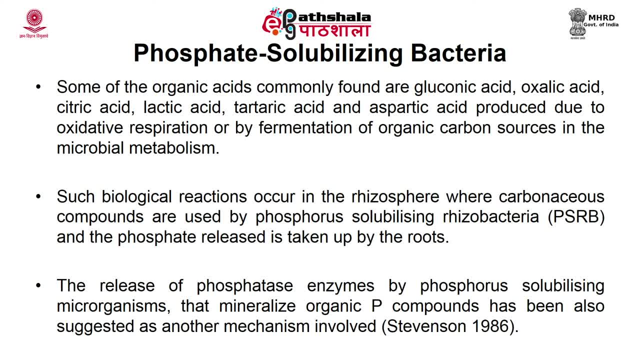 A very important: oxalic acid, citric acid, lactic acid, tartaric acid and aspartic acid, and these acids, they are produced due to oxidative respiration or because of the decomposition of organic carbon sources in the microbial metabolism. In addition to the above discussed mechanism, the release of phosphatase- 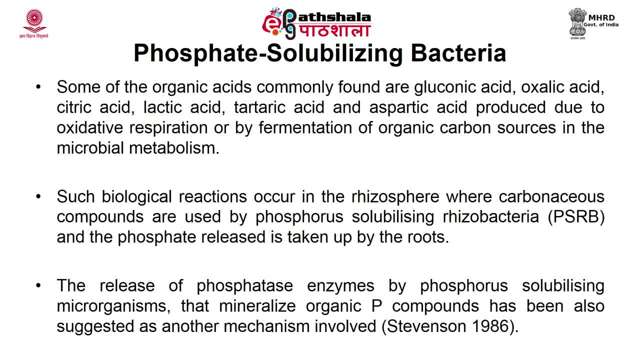 enzyme by the phosphorus solubilizing microorganism also mineralize the organic phosphorus compound and is also is the mechanism involved in the solubilization of phosphorus. So many studies have shown that inoculation of this group of microorganisms in the soil increases. 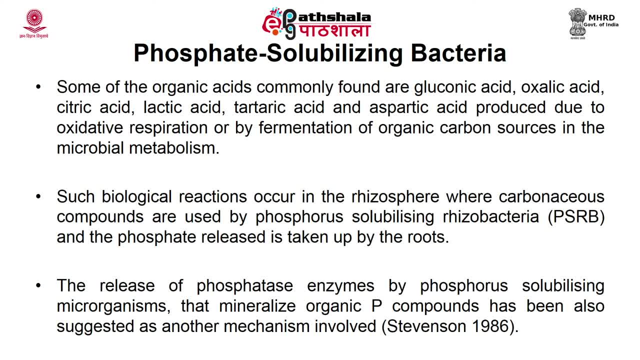 the available phosphorus content of the soil. Because of this property, only these phosphorus solubilizing microorganisms are produced by the phosphorus solubilizing microorganism, The phosphorus solubilizing bacteria they are forming. they are used in the agriculture as 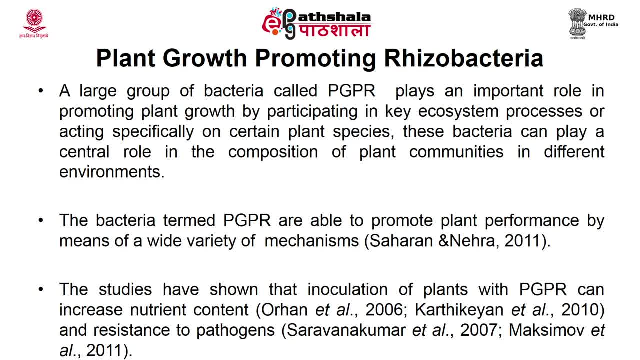 biofertilizers, Microorganisms also play a role of plant growth promoting rhizobacteria in the soil. This plant growth promoting rhizobacteria is a large group of bacteria which are commonly called PGPR, and they play important role in promoting the plant growth by different mechanisms. 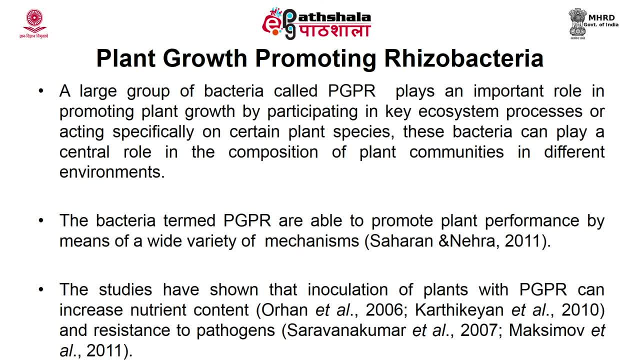 These PGPR microorganisms participate in key eco system processes act specifically on certain plant species and play a central role in the decomposition as well as in the composition of plant communities in the different environment. Moreover, some PGPR are able to produce � второй 수 head 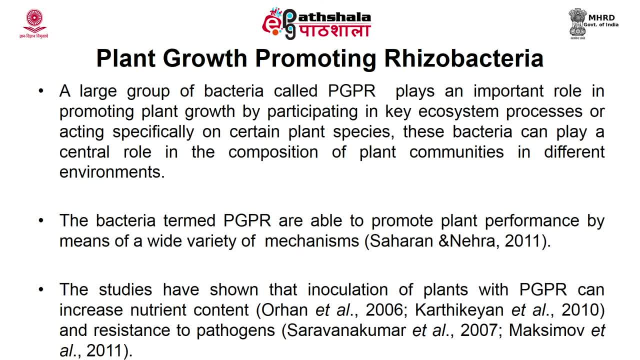 and control the population of harmful ones in the rhizospheric area of the soil. thus plants able to recruit greater population of these microorganisms into their rhizosphere and the this population is contributing for the better suitability of the plant. another community of the microorganisms, 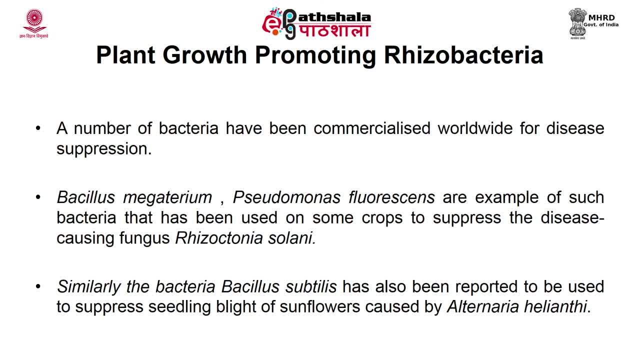 specifically bacteria present in the soil. they act as the disease suppressors. a number of bacteria have been commercialized worldwide for their disease suppression activity. this suppression is often very specific to particular diseases of particular crops and is effective in control of that disease, for example, bacillus magaterium, Pseudo monas, fluorescence and such bacteria. they 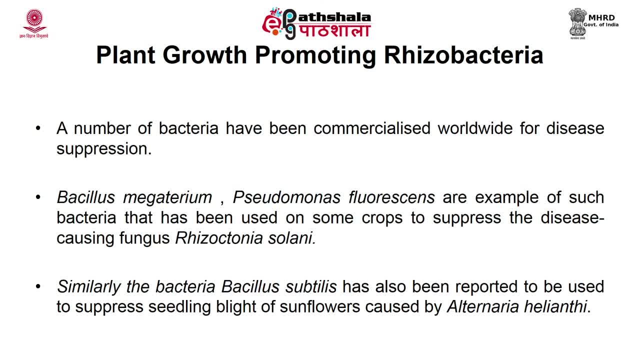 are commonly used in some crops to suppress their disease-causing fungus, the rice ochnia and, similarly, the bacteria which are present in the soil. as well as the bacteria present in the soil, bacteria, bacillus subtilis has also been reported to suppress the seedling blight. 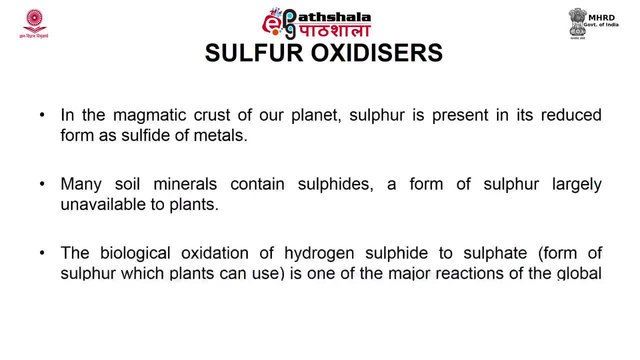 of sunflower caused by alternaria. another class of bacteria present in the soil belongs to sulfur oxidizers. these sulfur oxidizers: they are oxidizing the sulfide form of sulfur into sulfate, which is the available form to the plant. in the magmatic crust of our planet, sulfur is present in the reduced form as 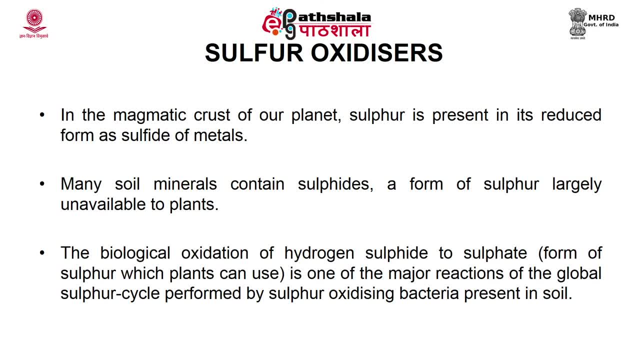 sulfide of metals, many soil minerals. they also contain the sulfites, and this form of sulfur is largely unavailable to the plants. the biological oxidation of hydrogen sulfide to sulfates by the microorganisms is a major reaction of the global sulfur cycle, and this action is performed by sulfur oxidizing. 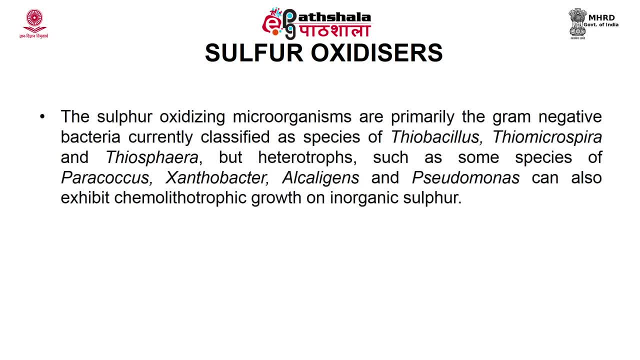 bacteria which are present in the soil. these sulfur oxidizing bacteria belong to gram-negative bacterial community and consists of the species thiobacillus and thiosaphira. they are heterotrophs, but some of the bacteria belonging to paracoccus, xanthobacter, alkyl genes and 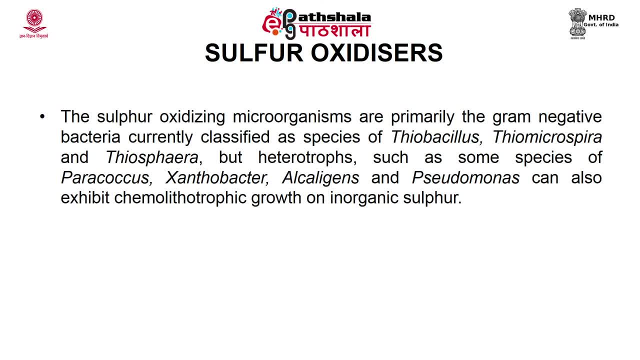 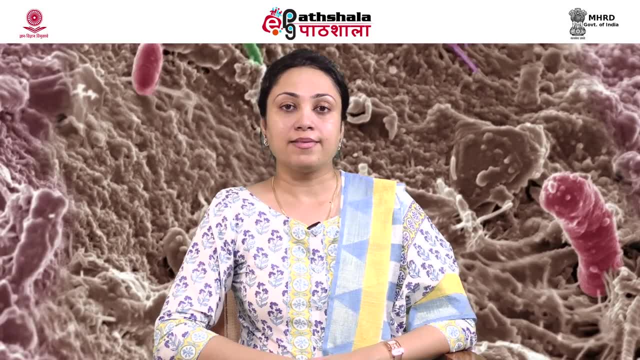 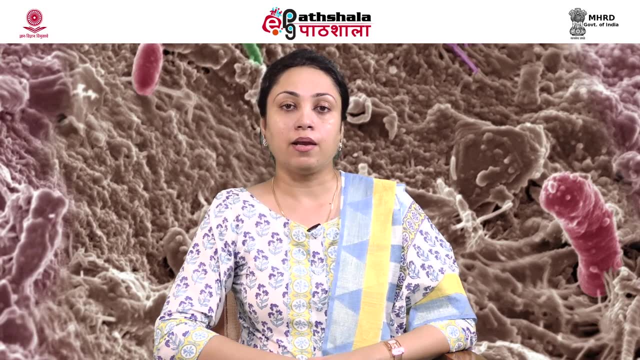 pseudomonas also exhibit chemo lithotrophic activity to oxidize the inorganic sulfur. to sum up this module, I can say that today, in this module, we have learned about the different kind of microorganisms which are present in the soil. in the soil they are playing a very